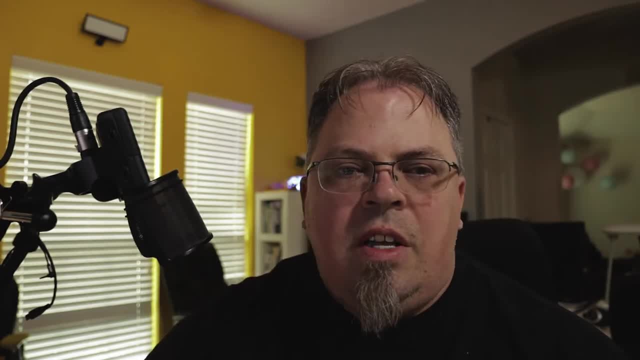 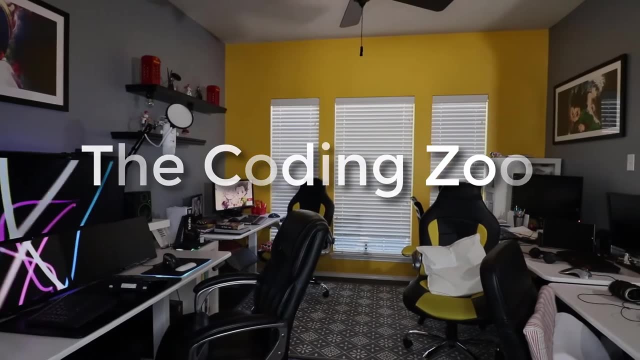 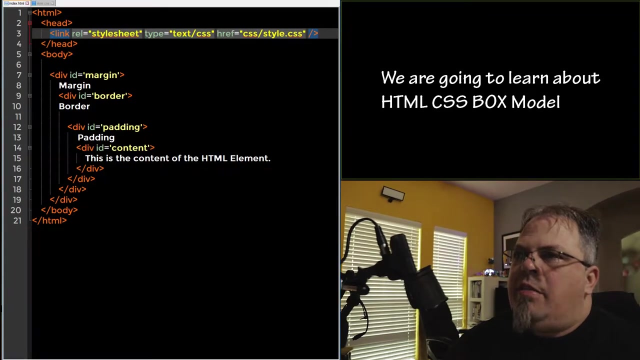 it's basically a model that wraps every element in html, so it's definitely something you have to know. i hope that interests you. if so, we're going to jump right in. all right, so hey, let's get started. um, so, on my desktop i have my index html file open. 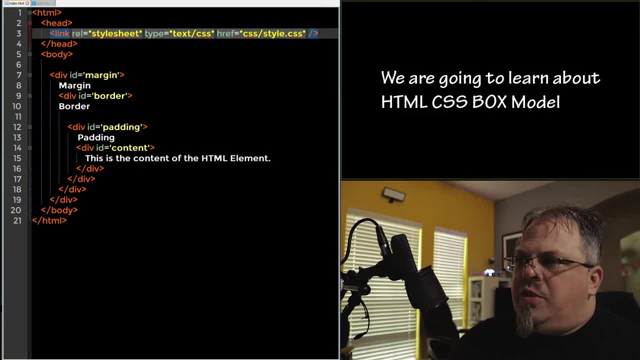 i have my style css file open. i definitely recommend that you try to program as i program. if you need to stop the video, go ahead and stop the video. if you can't, then hey, we'll have these files ready to download within a week or two. publishing this. 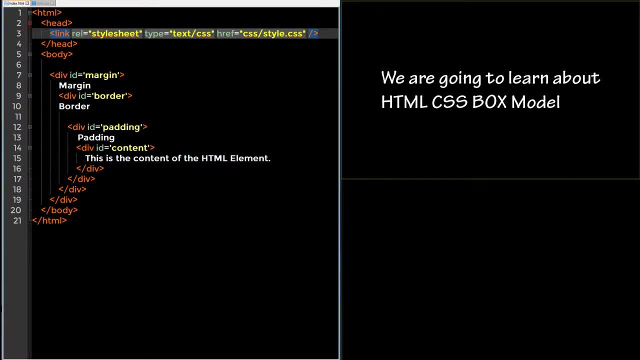 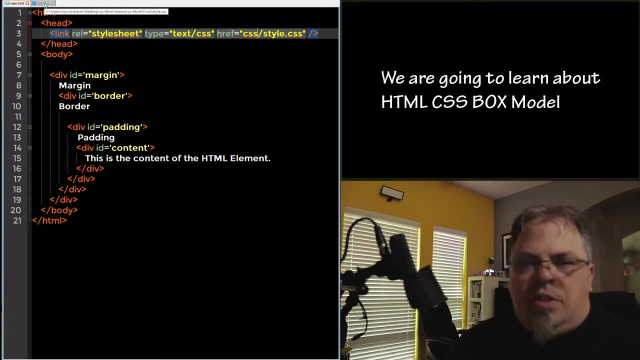 video on our website, thecodingzoocom. you can download the files from there and check it out. i went ahead and put together a couple of pages here just to demonstrate, uh, the html css block model. i put together a picture that should kind of give you an idea what that block model is. 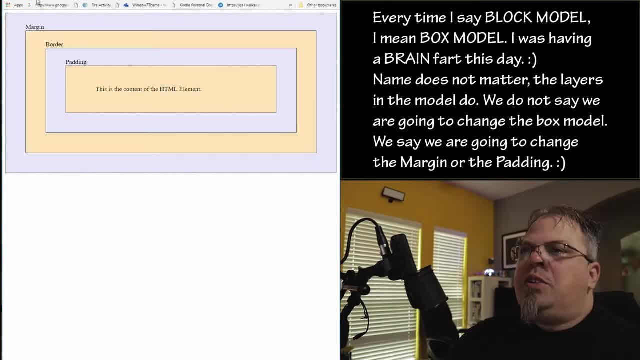 using this index and style sheet. let's go over to that page, let's refresh, make sure it's up to date. this picture is meant to show you the layers of that block model picture this content in the middle here, this square being a paragraph. it's, it's a few sentences wrapped in a paragraph. 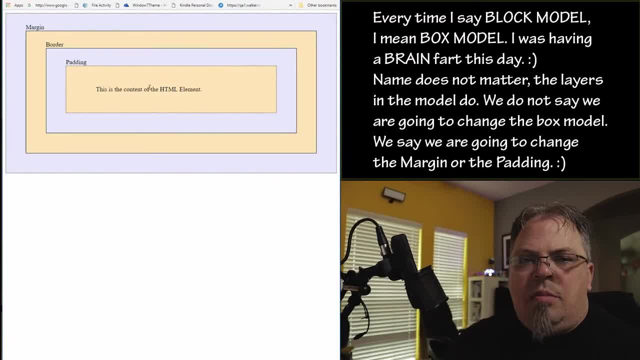 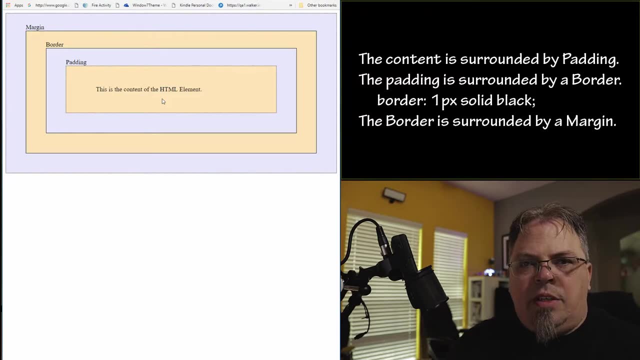 element. well, that paragraph element belongs to the block model. that paragraph element would wrap your content. picture this middle square being your content. well, on the outside of that content you'll find there is some space. that space is called padding and you can manipulate that padding to make other items be further away from your paragraph. that padding fits inside another. 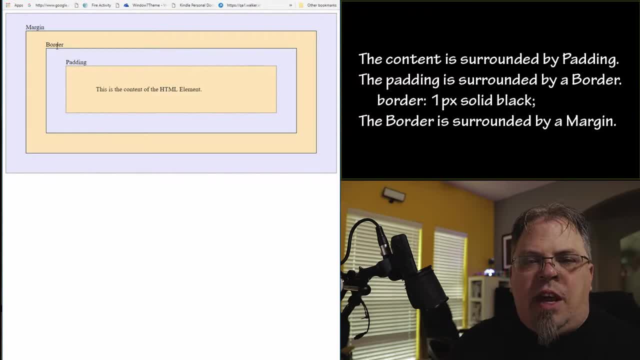 layer, which is your border. so your border is hidden. you can show it by using styles, and i'll show you how to do that in a few minutes. that border can be manipulated to be a dotted line, a solid line. you can change the style to whatever you like, but just just know that there is a 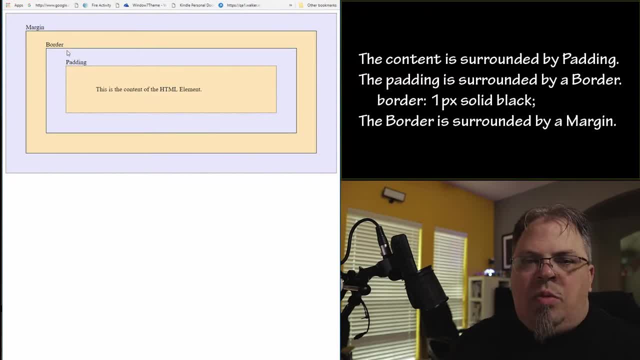 padding which is spacing around your content. there is a border and around that border is some more space. well, that space is called margin and again, that space can be manipulated to be smaller or larger, depending on your needs. your block elements wrap content. they have padding on the outside of. 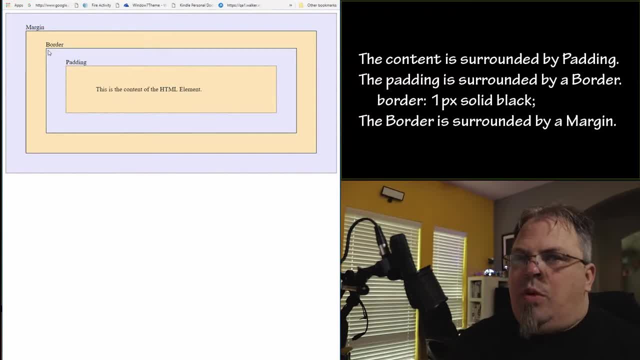 that content that's before the border. so the border wraps around the content that's before the border wraps around that entire block element and on the outside of that border is more space called margin. so those are the things you need to remember. you have padding on the inside, you have 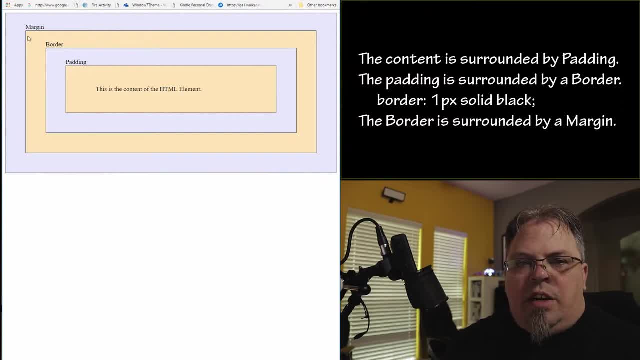 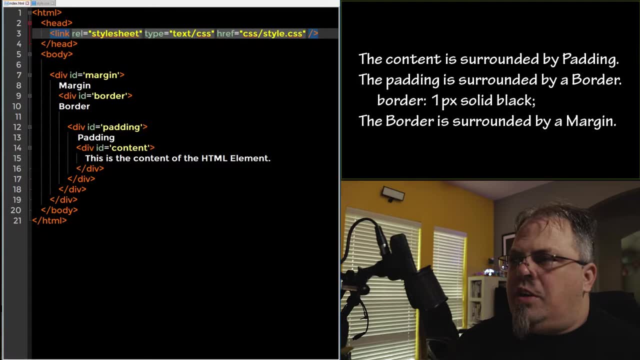 a border that wraps everything and you have a margin on the outside and you can manipulate all of them. let's jump in. i want to show you example of doing just that. i'm going to go back to my notepad, plus, plus over here. so, hey, let's real quick. let's add, uh, an element with some contents. 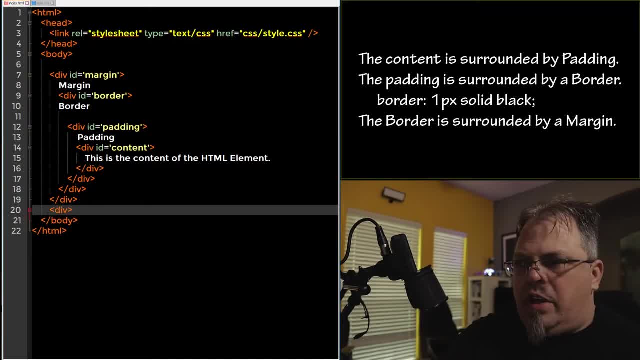 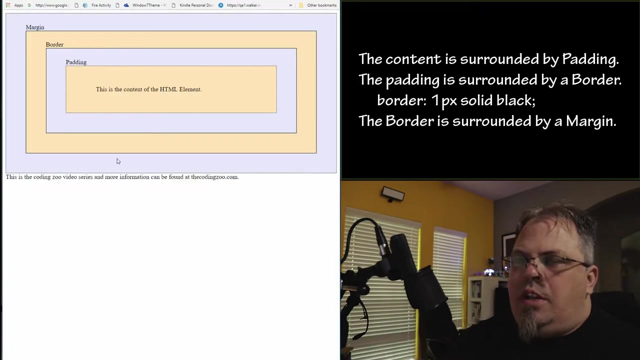 i'm going to add a div here and instead it could be a paragraph, could be anything i'm going to add. so all right, so i'm going to close my div. i have a sentence here. it's wrapped in a div element. let's go ahead and click save, click refresh, and there we go. so this is the coding. 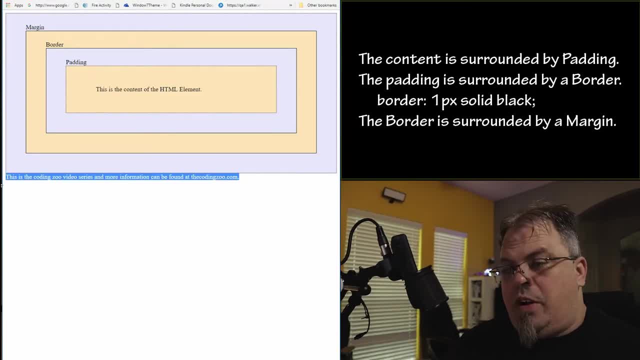 zoo video series and more about the coding zoo video series. i'm going to go ahead and show you here's the coding zoo video series and more about the coding zoo video series and more about the information can be found at thecodingzoocom. so this paragraph is wrapped in a div element. 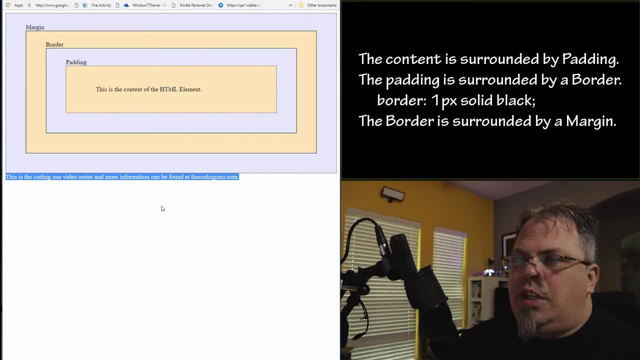 that div element has this model around it, so this is the content inside of that div. there should be padding on the outside of this, but if you look at it well, there's not much space there, so i think the padding is probably set to zero. uh, there's no border and there's no margin. 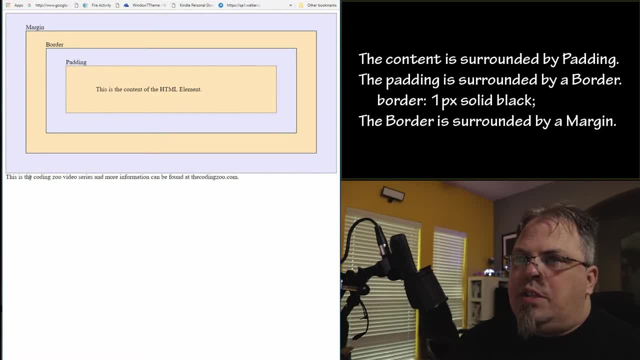 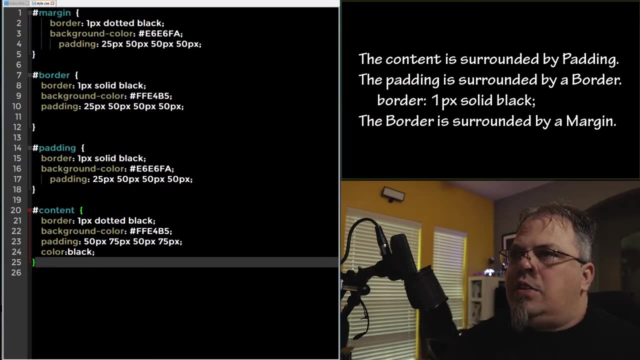 so you can't really see the border. and again, there's no space here, so there's probably no margin either. let's go ahead and fix that and we can show you how to change all of these items. jump over to css here, let's. let's go back and give this div an id. 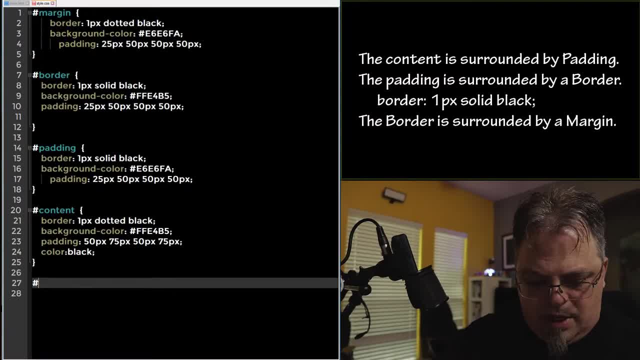 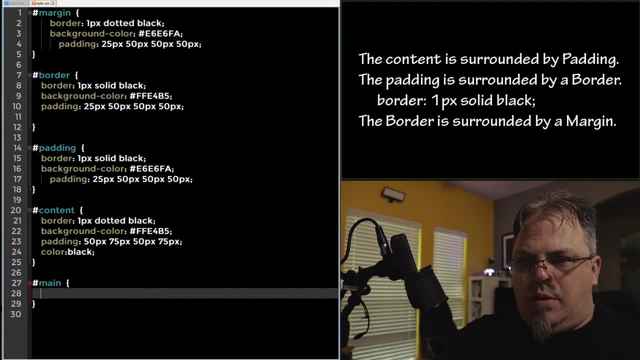 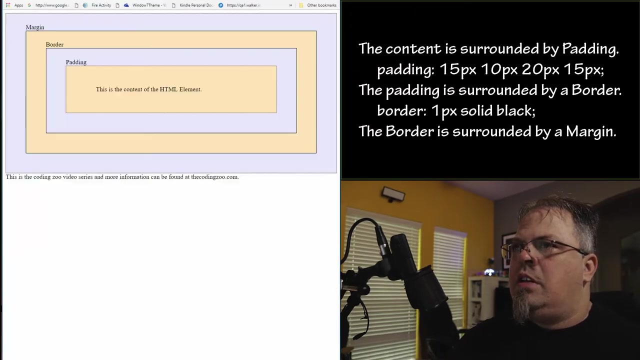 all right, so i gave the div an id. we're going to access it with the name selector. id selector called it main. okay, i want to first add a border so we can see that div. all right, all right, so you'll notice now it has a block around it. this is my border. i just activated it. 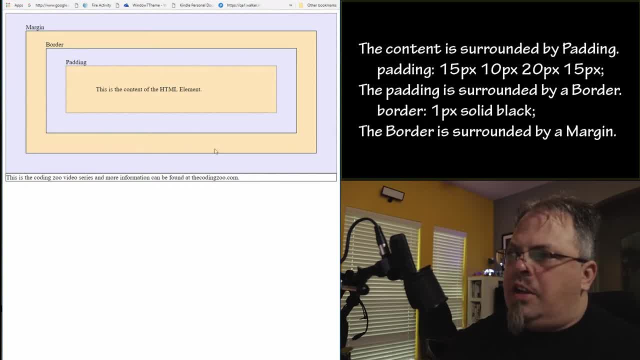 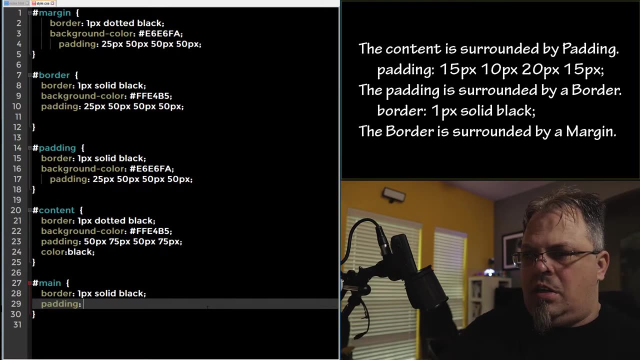 if you look this model up here, see how this block here that is meant to signify your border. so between your border and the actual content there should be some padding. there's not, must be set to zero. let's go ahead and change that. all right, so i added padding: 10 pixels. 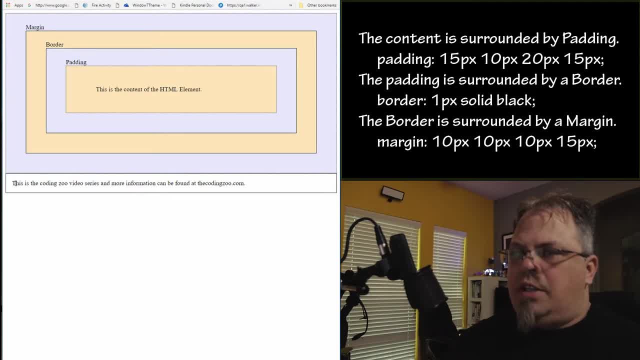 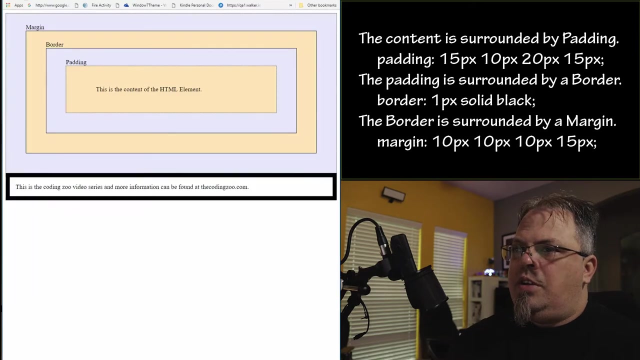 refresh. there we go. so now i have the content which is signified here. here's the content. there's padding around it, so you see the space around the content and there's a border around it, so you see the line going around. that's your border. keep in mind, i can make that border as large as i want to. of course, there's usually no need to. 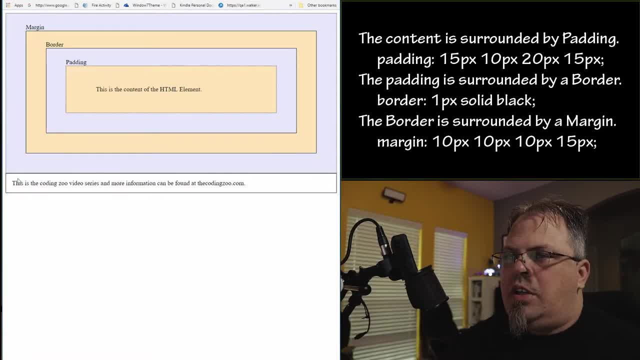 so you'll notice the border here. i've got padding between my content and the border, but my border here is right up on this other picture up here. it's right up next to this other border. i don't have a margin. the margin again must be defaulted to zero with this div. 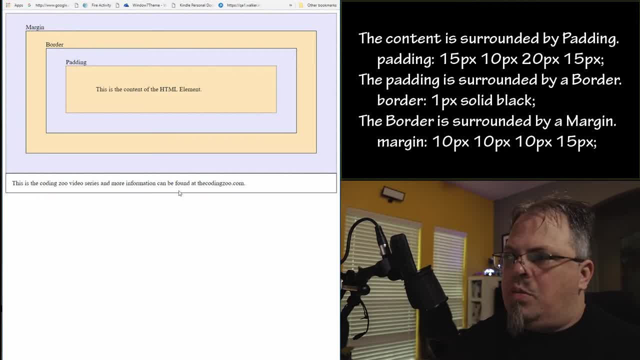 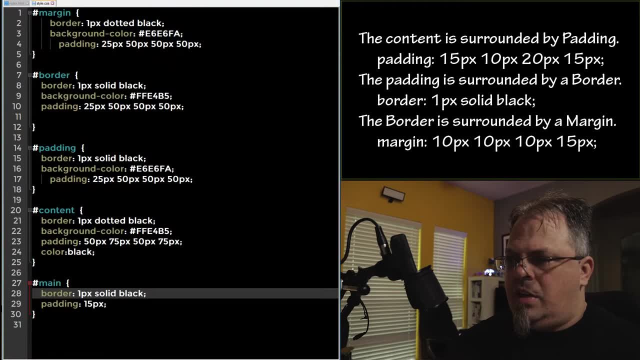 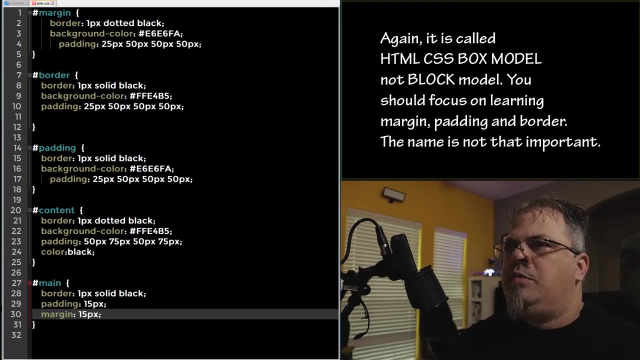 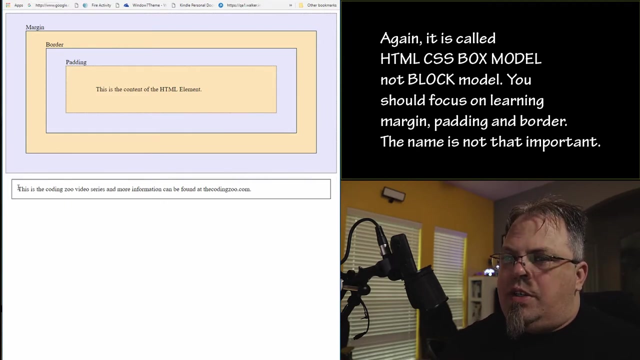 let's go ahead and fix that. what we should see is this whole block element should be separated from this picture up here. all right, so i'm at a margin, click save, click refresh, and that should push away from the other element. there we go. so i added 15 pixels on. 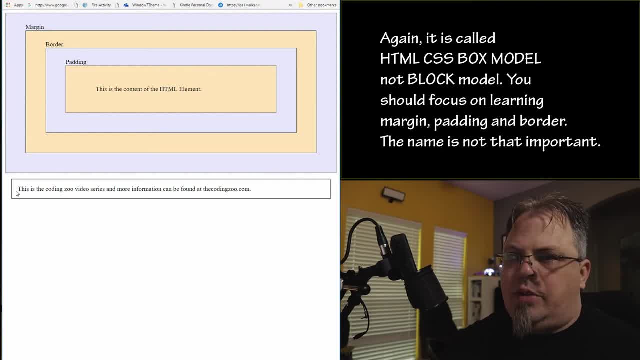 each side. you'll notice, as i set a pixel size for margin for padding, that it did it all the way around the block element. so there's 15 pixels on each side. so i have a margin here of 15 pixels. i have a border that's one pixel wide and i have padding on the inside and in the middle is my. 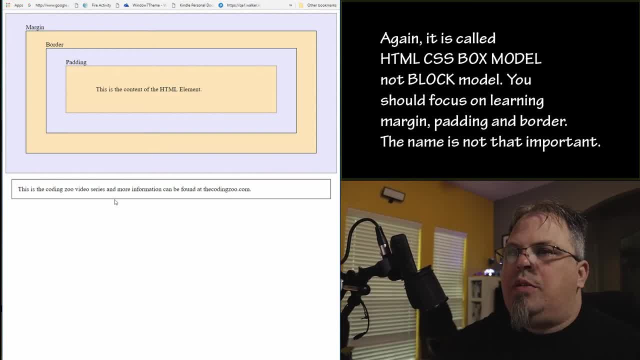 content. that's it. this is the hml css block model. it's very important to understand how to manipulate this model so you can move things around, space them correctly, make your web page look good. so you definitely want to learn this model. you want to learn a difference in padding and margin.